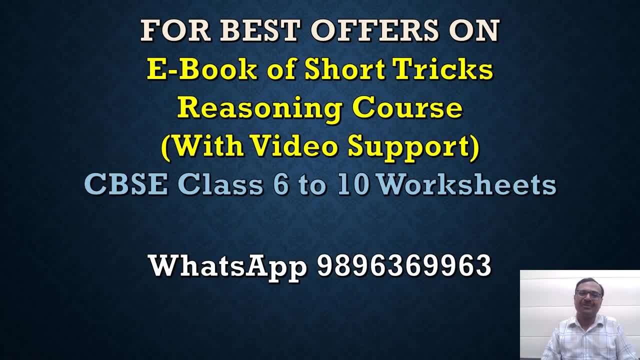 yes, you are a champion, prince. we have the festive season going on and on the occasion of this upcoming the shara and divari, we have the best offers on the ebook of short tricks, the reasoning course which comes with video support, the combo. the cost is going to surprise you. it's not five. 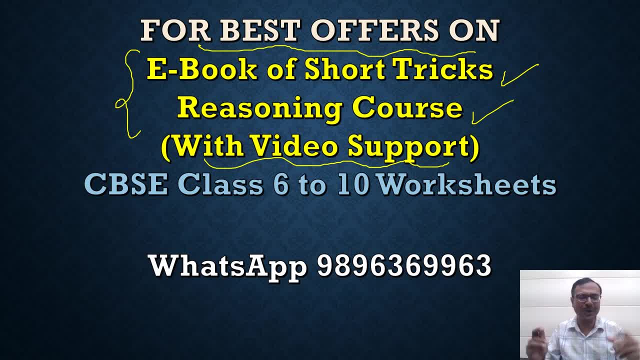 thousand, it's not ten thousand, it's like very nominal- and therefore i advise you to go for the ebook of short tricks and the reasoning course, which will help you in developing 10 times faster speed of calculations, because it gives you 350 different short tricks of 24 topics, that is. 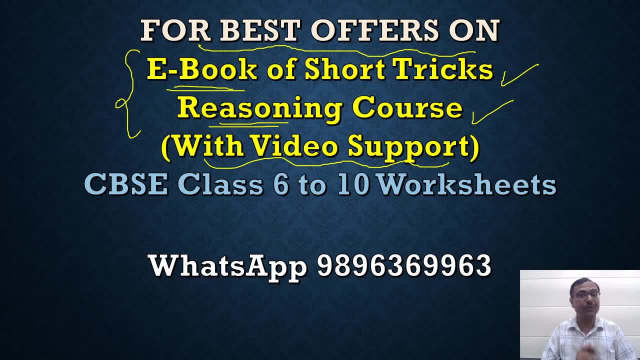 quantitative aptitude: 15 topics of reasoning with video support. you don't understand anything. watch the video and you will understand everything. for cbsc students that you this channel is, you know, providing exclusive content in the form of class 10th, 6 to 10th. 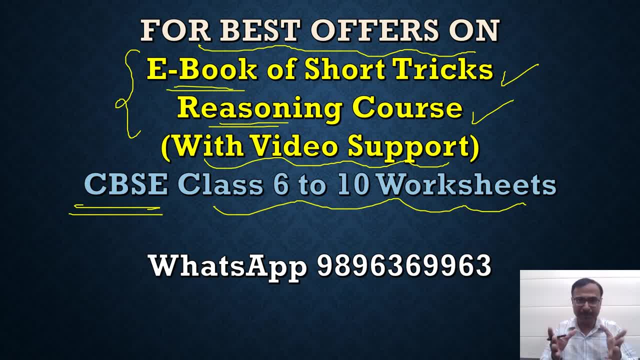 worksheets. these are exclusive worksheets specially made for the cbsc students so that they can excel themselves. they can test themselves and practice all those important concepts. and these worksheets are not available anywhere on the internet or in any print form, in any book. go for it. whatsapp. 9896369963. 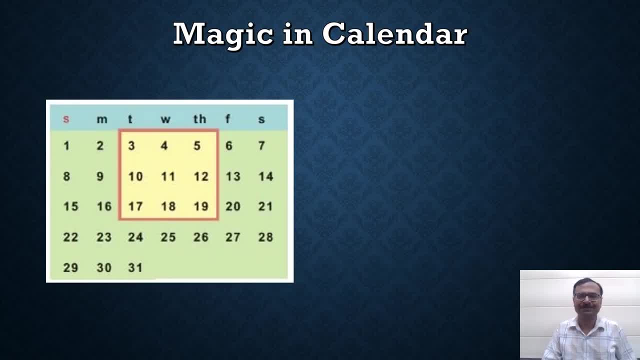 now let's see the magic in hand now. so calendar, right. so i picked up a random calendar there: sunday, monday, tuesday, wednesday, thursday, friday, saturday. so what is so special about this if you pick up a three by three matrix from this calendar, just like i have already put a square? 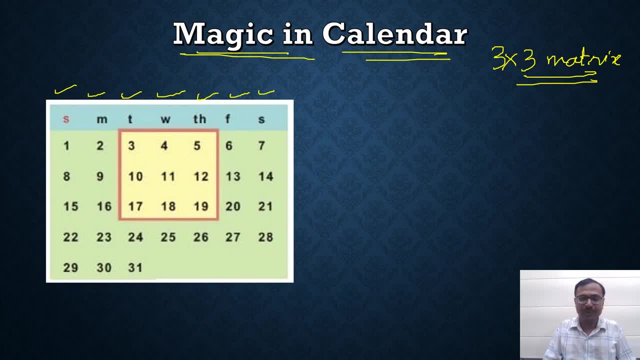 there. so if you see three, four, five in the first row, 10,, 11,, 12 in the second row and 17,, 18,, 19 in the third row, The special thing is, which is the smallest number I have picked up? The smallest number is 3, and what do you do with? 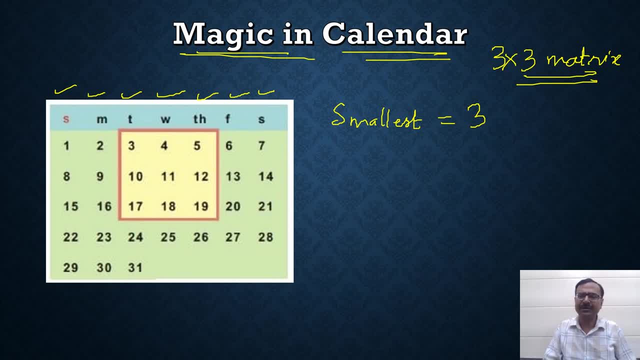 this 3?? Just try and add 8.. Now, this is a default number. You have to add 8 only, okay, to the smallest number. So 3 plus 8 will give you 11, and then multiply this result by 9.. 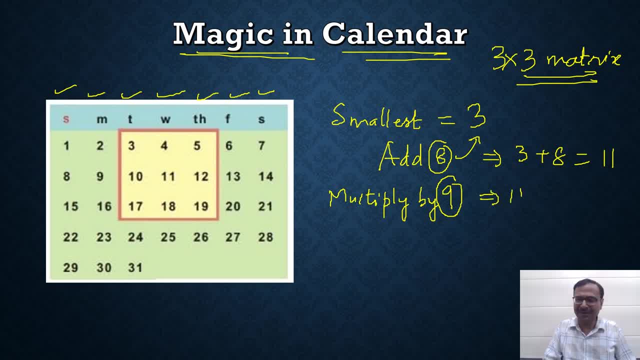 This is also a default number. So 11 times 9, that's 99. but how does 99 relate itself with the matrix which I have marked there? Let's add all the numbers which I have put together. So let's add all the numbers which I have put together. So let's add all the numbers. 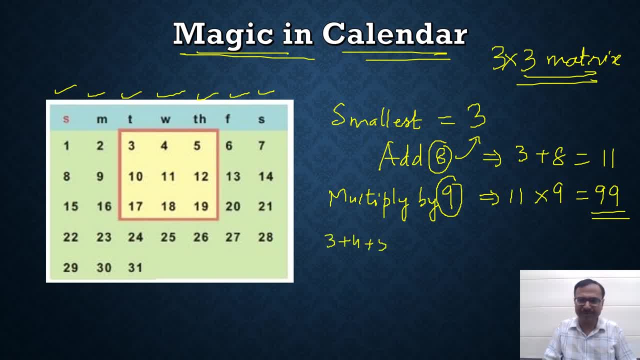 in the square: 3 plus 4 plus 5, that's the first row. 5 plus 4,. 9 plus 3, 12 right. 10 plus 11 plus 12, that's the second row, that's 33 and the third row 17 plus 18 plus 19.. How much is that? 35, 45,. 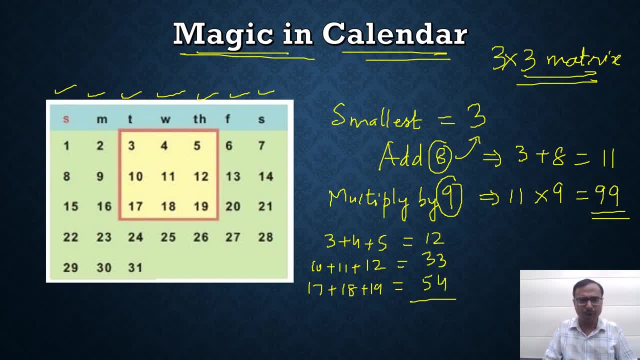 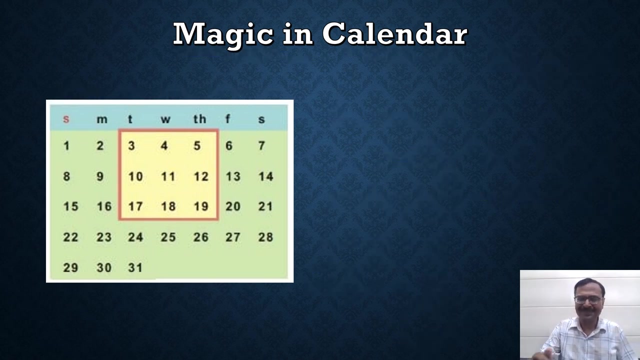 55, 54, right, Let's add all nine numbers: 99.. Oh my god, I got the same number as the sum of all nine numbers. Friends, that's really, really amazing, right, But is it universally applicable to all calendars? Let's try taking some other matrix in the same calendar. So here we have the 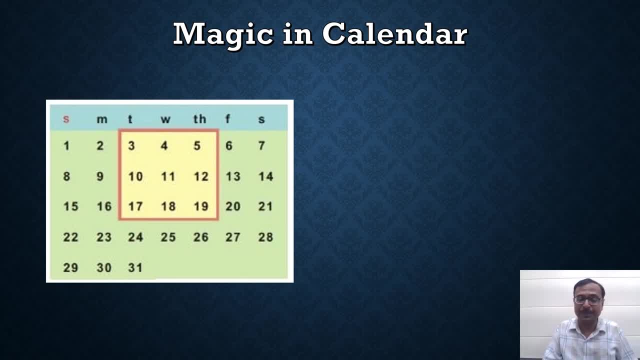 same calendar again, and now I'm going to pick up some other nine numbers. So let's pick up the matrix here. So I'm encircling it so that we can distinguish it from the previous matrix which we have taken up Now. this is the matrix I am taking up Now. in this matrix, the smallest number. 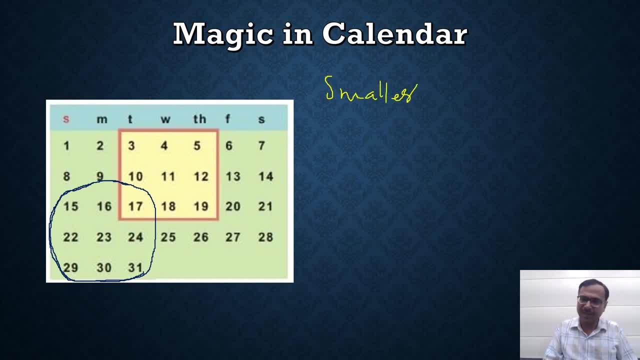 which I can see is 15, and I told you, add 8 to this, you get 23, and then multiply by what- 9.. So this is 207.. Now let's check the sum of these numbers: 15 plus 16 plus 17, the first row.